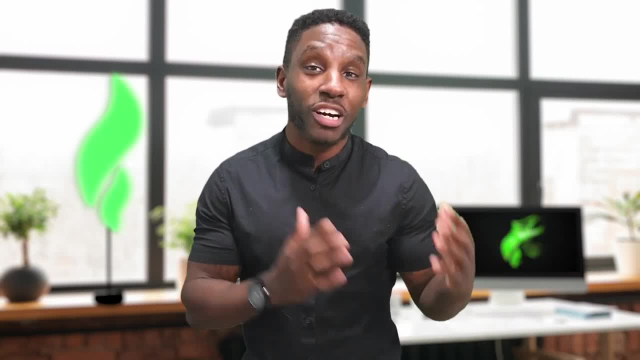 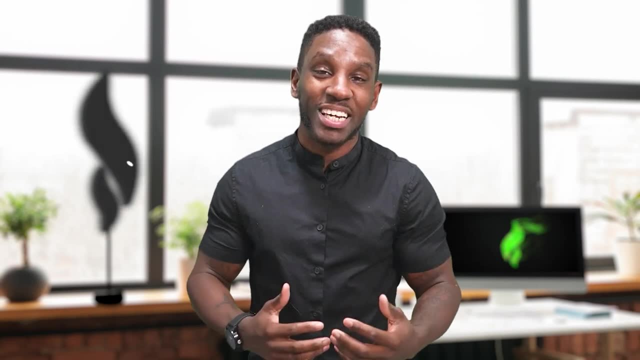 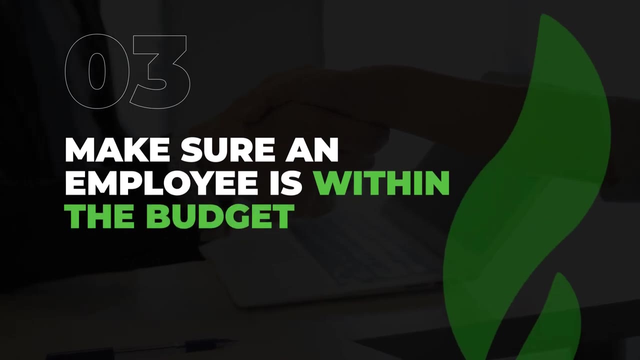 it by now. In short, the reason you will hire an employee over a contractor is because of the relationship it provides you. You are willing to take on the extra responsibility in exchange for loyalty and control. Step number three: make sure an employee is within the budget Look. 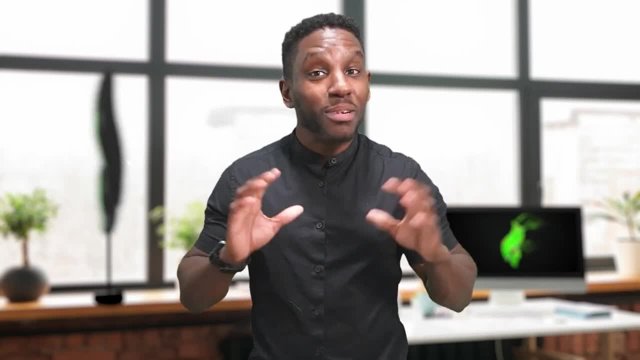 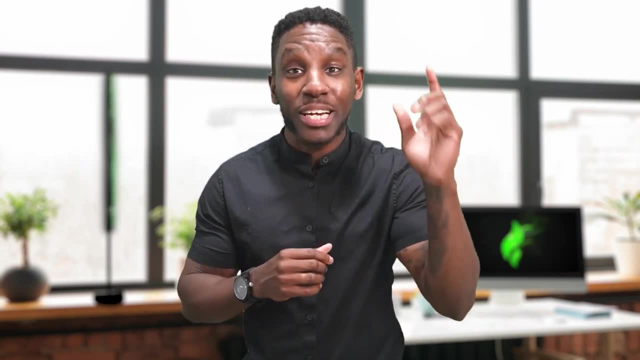 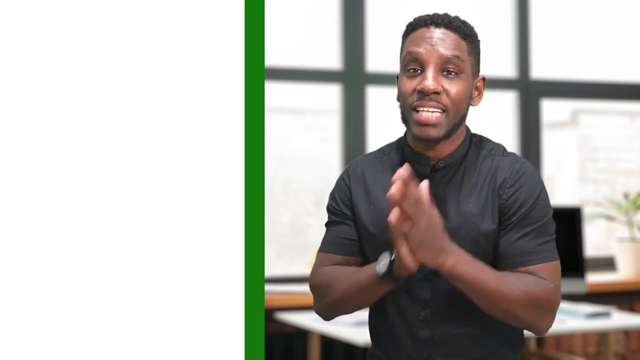 I've seen many business owners make a huge mistake. They believe that the true cost of an employee is the employee's hourly wage or salary and completely forget about all of the other costs that come with having an employee. Of course you have their wage. This includes the 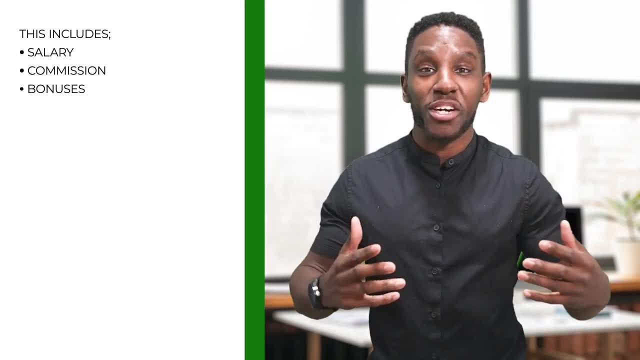 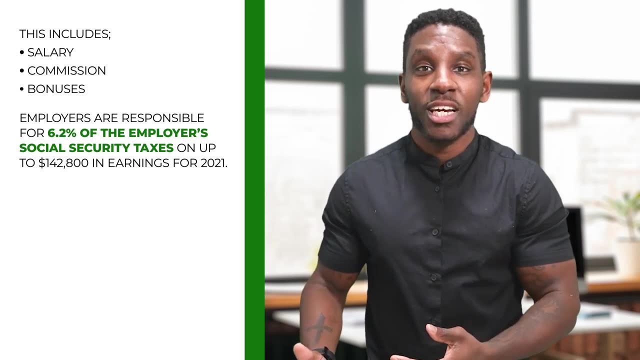 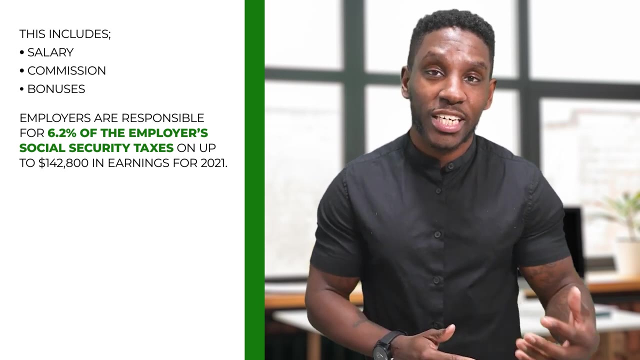 salary commission and bonuses, But then you have federal payroll taxes on top of their wages. Remember, employers are responsible for 6.2% of the employee's social security taxes on up to $142,800 in earnings for 2021.. Oh, and don't forget Medicare taxes. 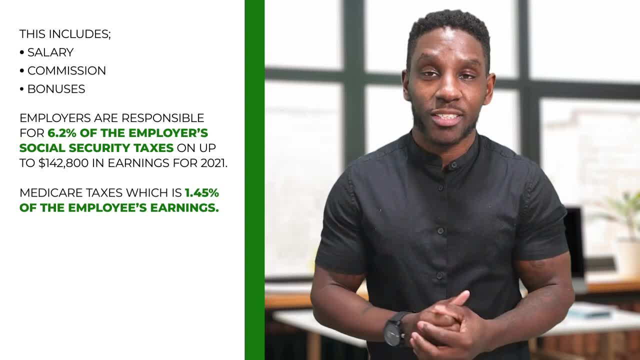 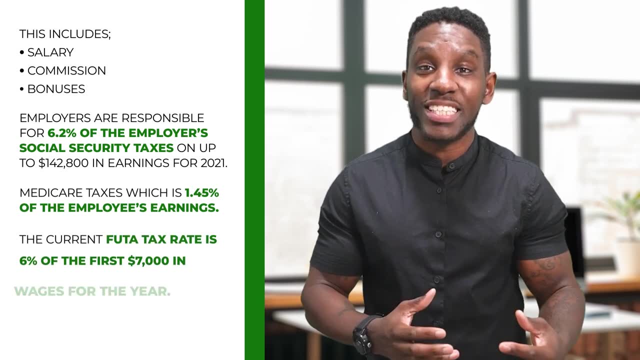 which is 1.45% of the employee's earnings. You also have to pay FUTA taxes as an employer, which stands for federal unemployment taxes. The current FUTA tax rate is 6% of the first $7,000. in wages for the year. Some states also require that you pay unemployment taxes at the state level. Then some states require that you pay unemployment taxes at the state level. Some states require you to have workers' compensation insurance after a certain number of employees, And the best part about it all is that we haven't even begun to talk about. 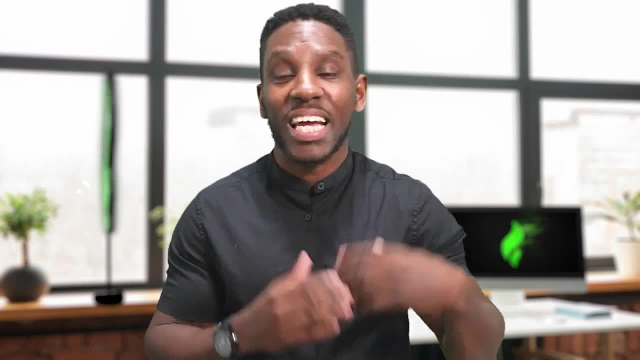 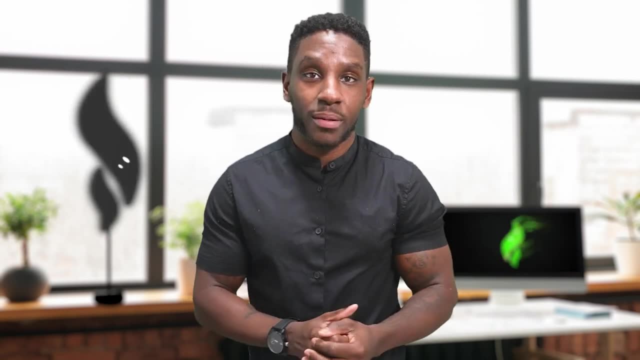 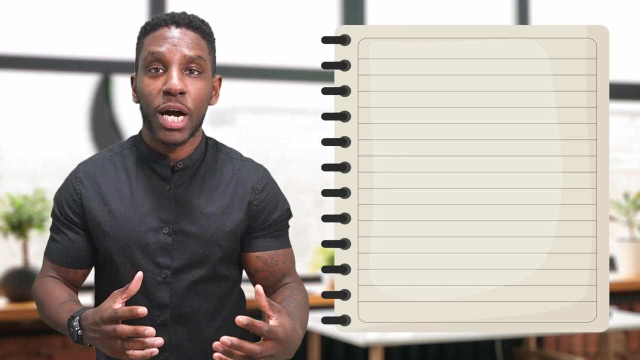 the cost of providing benefits, PERC, supplies and space. So, as you can see, the true cost of an employee doesn't end at the hourly wage and salary. Step number four is to create an employee handbook and standard operating procedures. Your employee handbook helps. 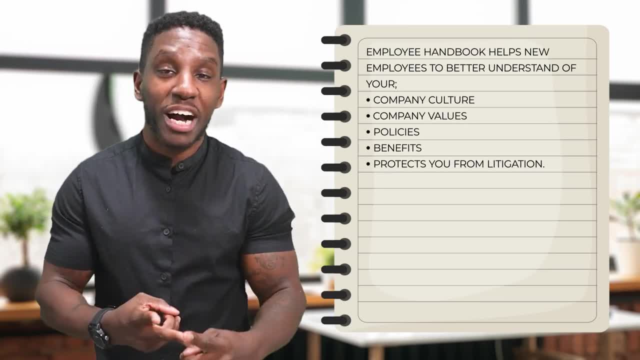 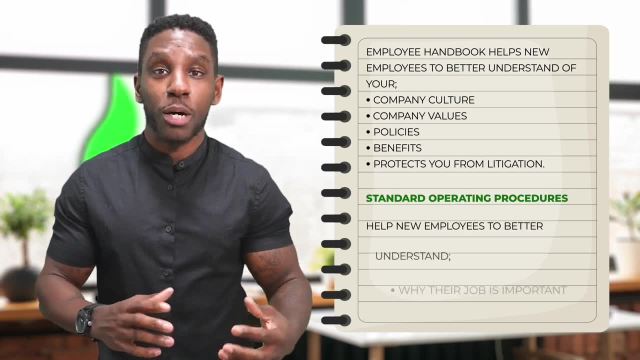 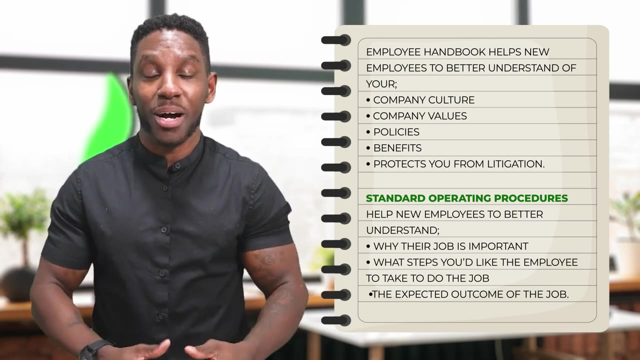 new employees to better understand your company culture, company values, policies, benefits and simply protects you from litigation. Standard operating procedures help new employees to better understand why their job is important. what steps you'd like the employees to take to do the job and the expected outcome of the job. 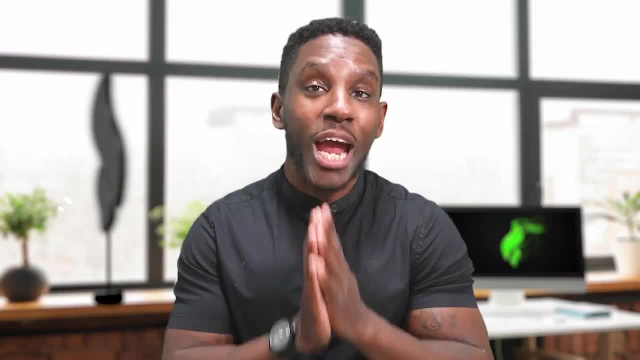 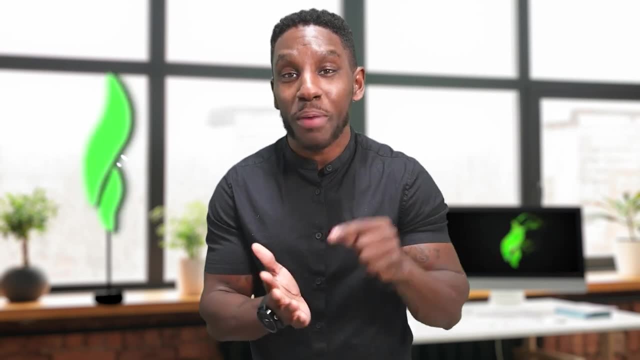 You should have an SOP, a standard operating procedure, for every possible task in your business. If you think it's common sense, trust me, it isn't until it's on paper. Together, the employee handbook and standard operating procedures help new employees to better. 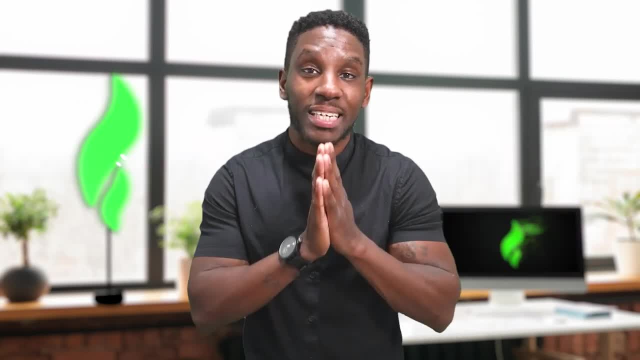 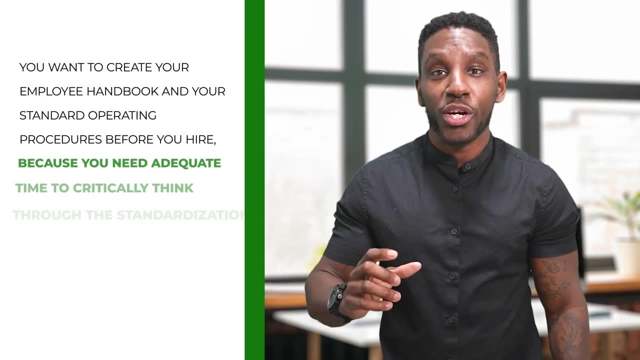 understand their job. The employee handbook and SOPs help to standardize and systematize your business. You and your employee both know what is expected. Now, ideally, you want to create your employee handbook and your standard operating procedures before you hire, because you need. 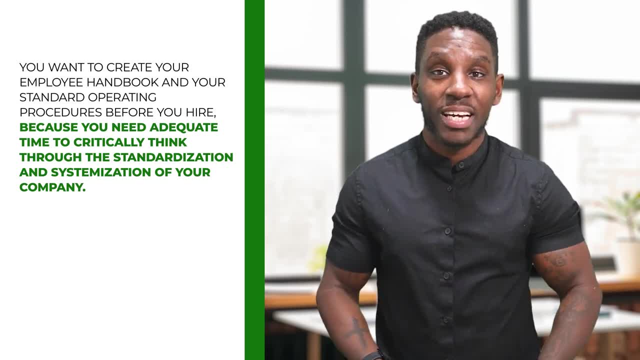 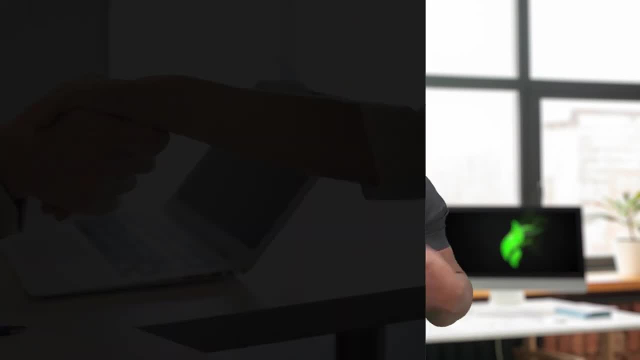 adequate time to critically think through the standardization and systematization of your company. Okay, now it's time to get into the process of hiring an employee. Step number five: create a job description. Now, I'm not going to tell you how to do that, but I'm going to tell you how to do that. 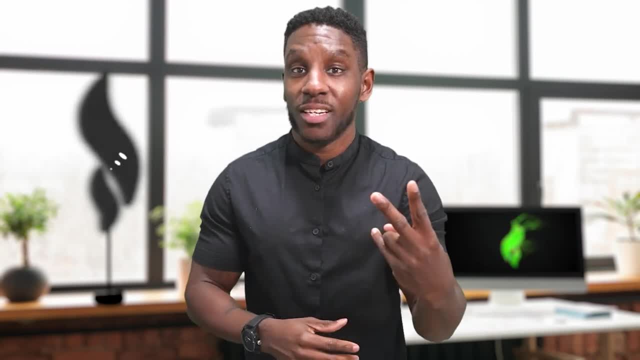 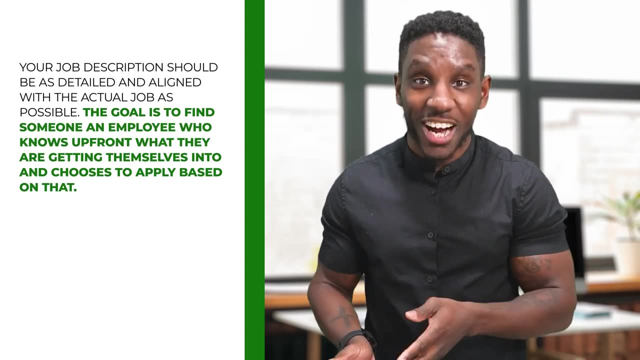 I don't want to spend too much time here, but I do want to tell you two things when it comes to your job description. First, your job description should be as detailed and aligned with the actual job as possible. Your goal is to find someone- an employee- who knows up front what. 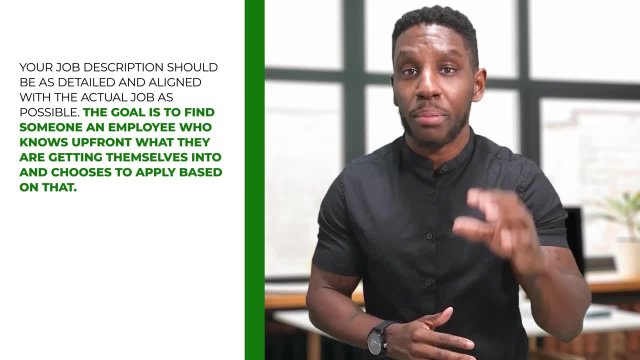 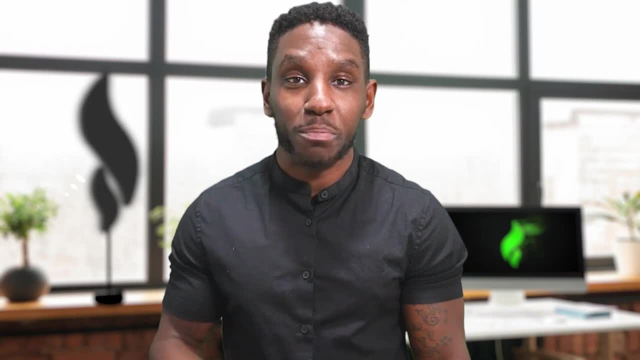 they are getting themselves into and chooses to apply based on that. Look, the last thing you want is to waste your time in interviews with people who are shocked by the duties and responsibilities of the job. Secondly, you want to find someone who knows what they are getting themselves into. 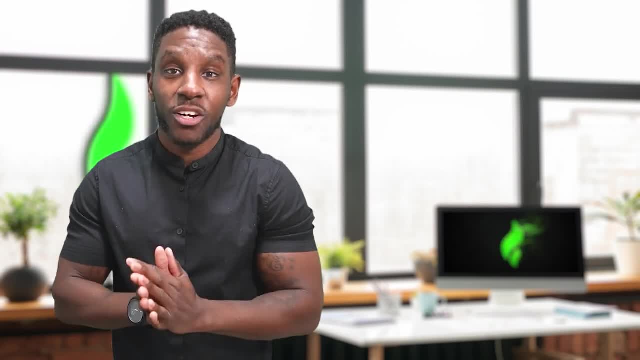 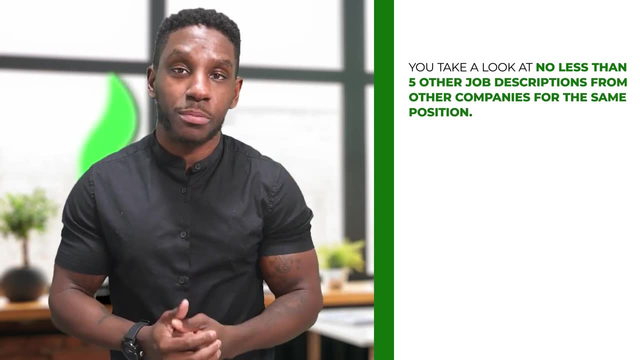 unless the position you are hiring for is extremely unique or you are a wizard at copywriting, I would suggest that you take a look at no less than five other job descriptions from companies for the same position. Not only will you start to understand what your job market competition. 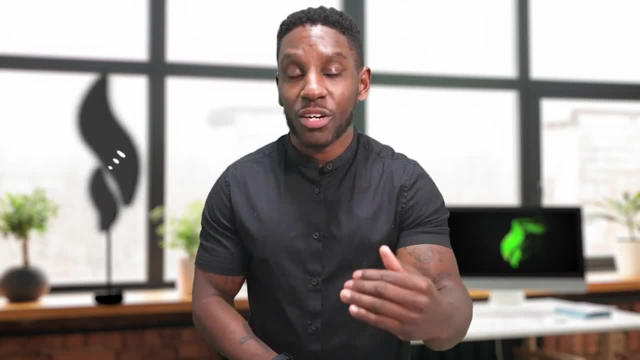 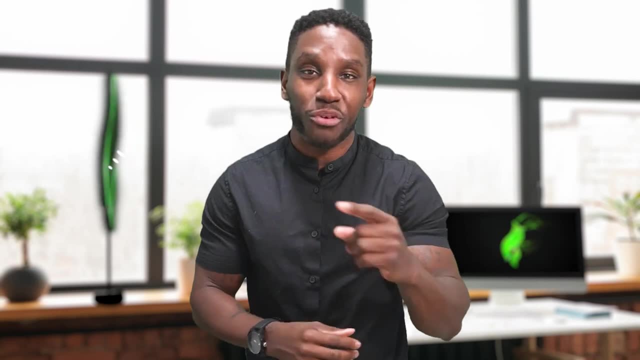 is offering, but I guarantee you will find a clearer way to express the job duties within your own description by taking a sneak peek at what others have written. Step number six: create a system for hiring an employee who knows up front what they are getting themselves into. 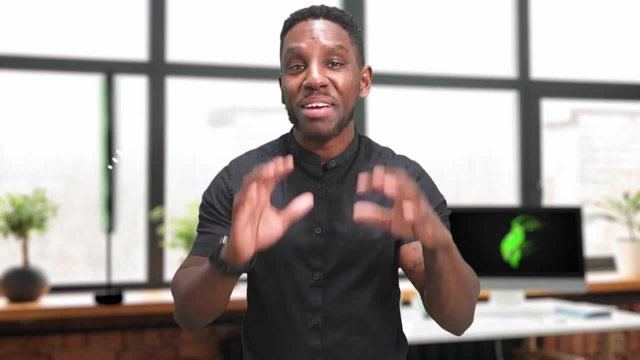 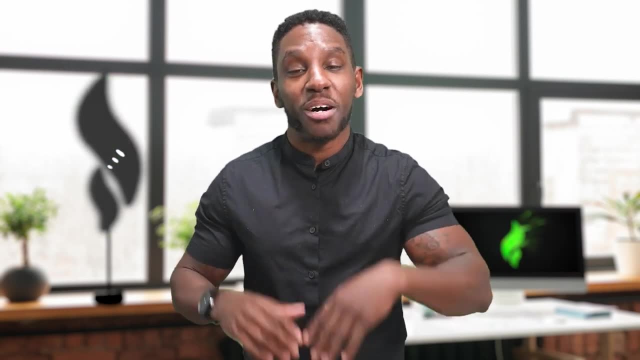 Step number seven: create a system for identifying top talent. Nothing- and I mean nothing- is worse than hiring someone you believed was going to get in the role and crush it, only for them to become a nightmare employee. I've definitely had my fair share of that in the past, but lately I have truly. 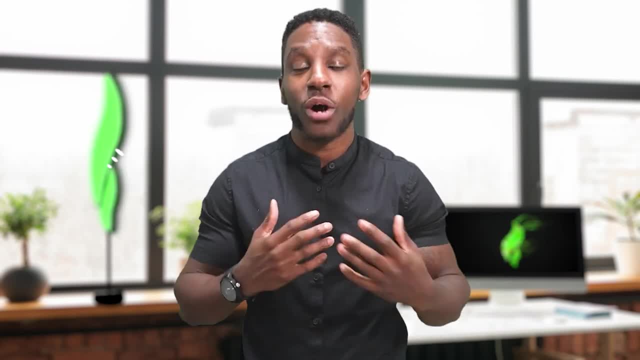 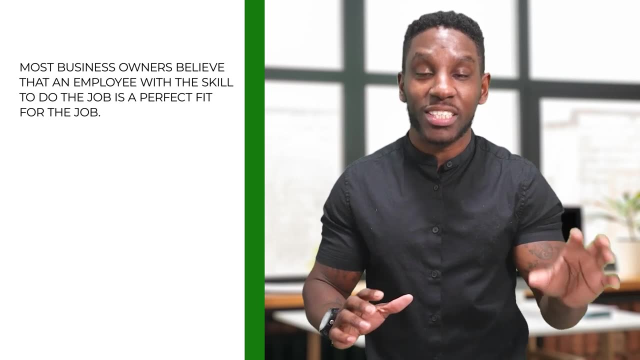 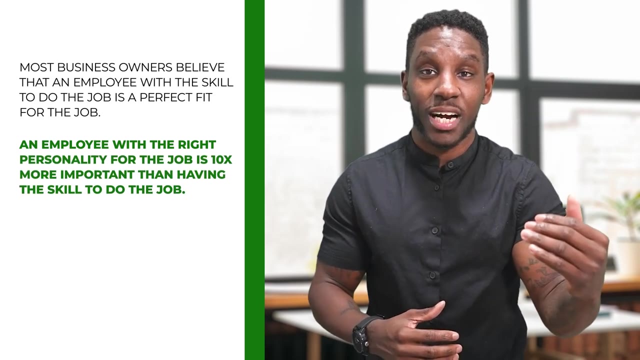 dialed in on what we consider top talent for our business, And it's not what you think. You see, most business owners believe that an employee with the skill to do the job is a perfect fit for the job, But I'd argue that an employee with the right personality for the job is. 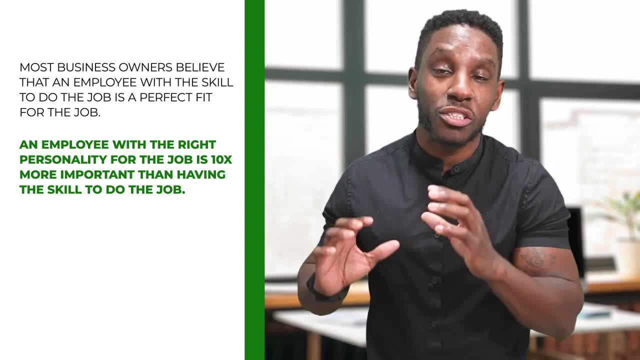 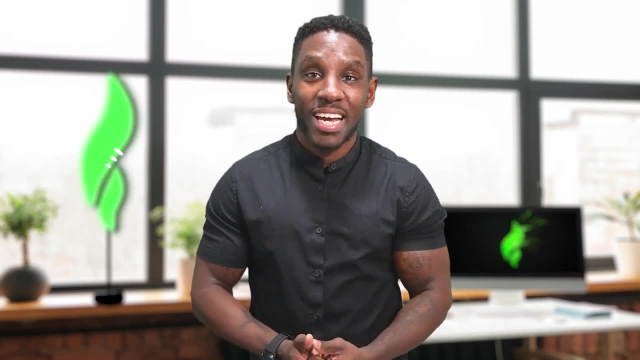 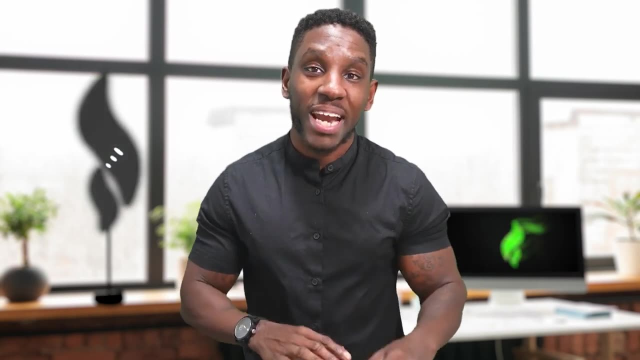 ten times more important than having the skill to do the job. Once my team and I switched to skills only being a prerequisite to your resume being looked at and a personality fit a requirement to get an interview, we seen our employee turnover drop dramatically and employee satisfaction increase. We currently use a program called 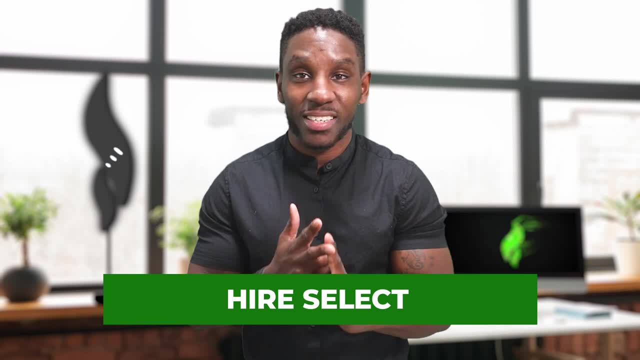 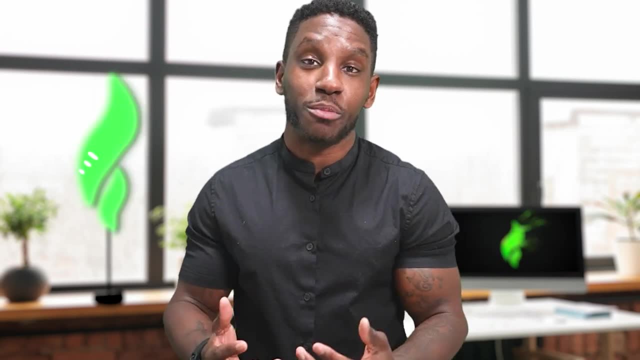 HireSelectcom. HireSelectcom is a great place to find out more about your employees, applicants, aptitude, personality, emotional intelligence and skills. It's simply been a game changer for us and happy to share with you entrepreneurs so you can find the best candidates. 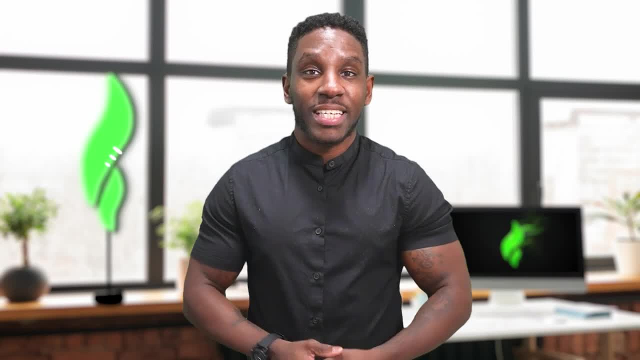 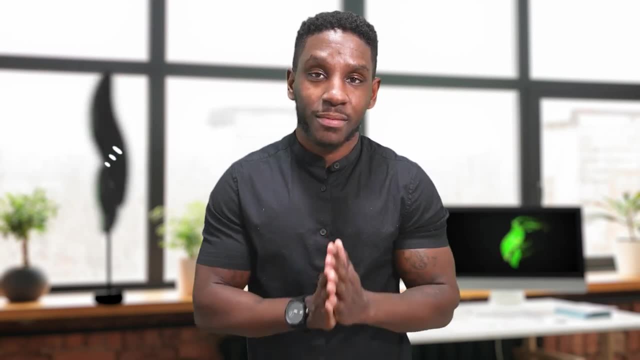 All right, let's talk about what happens after you make the hire. So you found your ideal candidate, they've reviewed and signed their employee contract, and their start date is approaching. Here's what I want you to do. next Step, number seven: check workers' compensation insurance. before. Different states have different requirements for workers' compensation insurance. For example, here in Georgia, most employers with three or more full-time, part-time or seasonal employees are required to have workers' compensation insurance, And if the business is incorporated or an LLC, the corporate officers or members are included in the three or more employee. 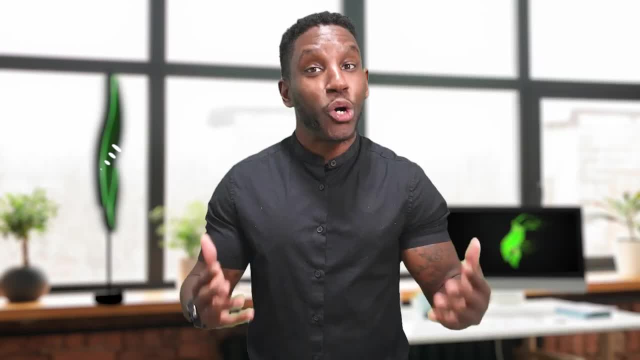 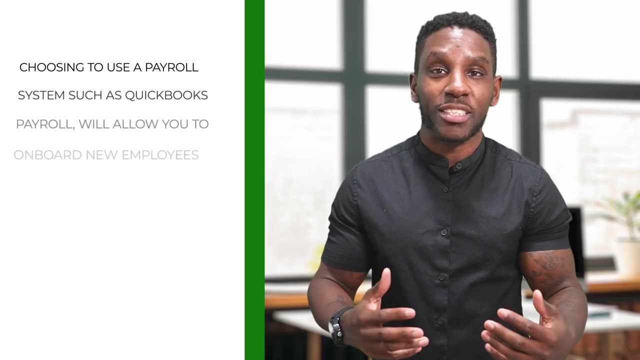 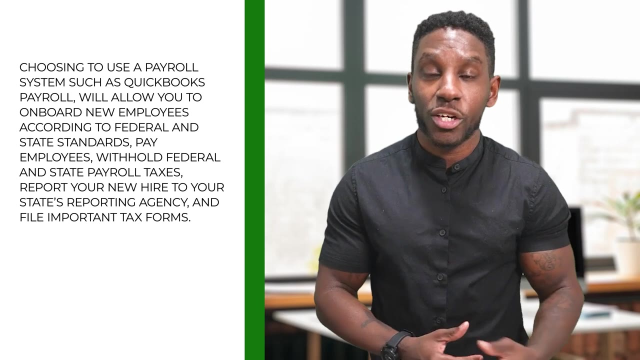 count regardless if they exempt themselves from coverage, So be sure to check your specific state requirements. Step number eight is to set up payroll. Choosing to use a payroll system such as QuickBooks Payroll will allow you to onboard new employees according to federal and state standards. 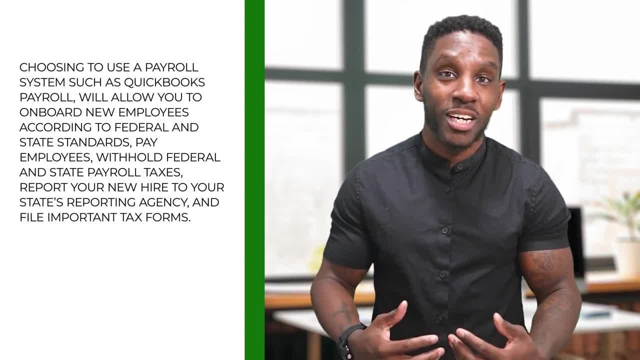 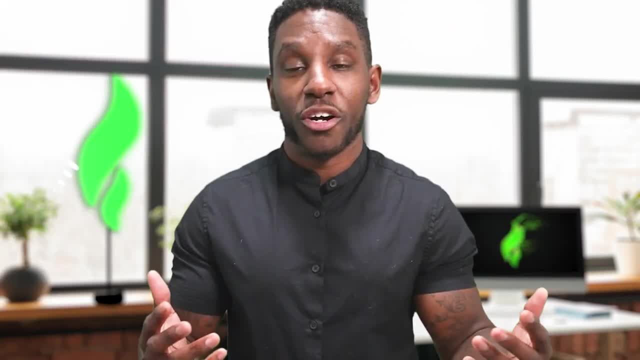 pay employees, withhold federal and state payroll taxes, report your new hire to your state's reporting agency and file important tax forms. Now don't get me wrong. you can attempt to do this manually, but saving a penny could cost you thousands in mistakes. 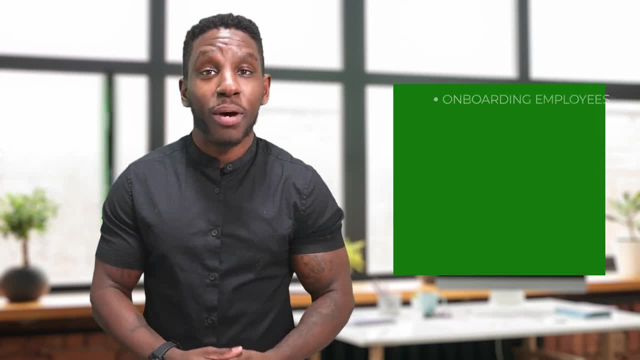 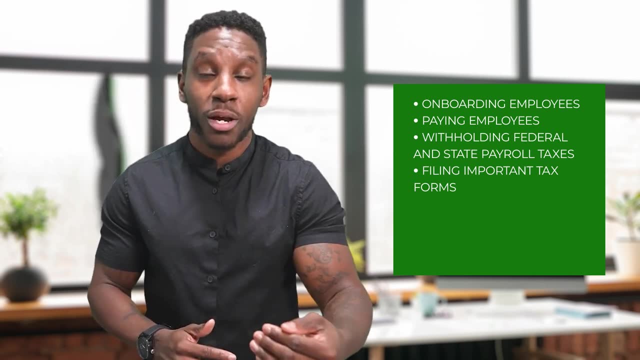 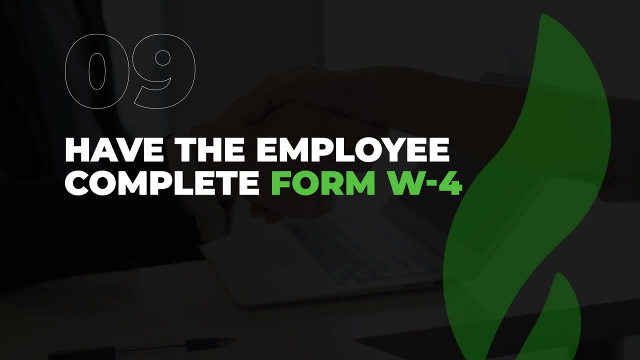 of time. So for this reason, use a payroll system to make the process of onboarding employees, paying employees, withholding taxes and filing important tax forms easy, accurate and automatic. Step number nine: have the employee complete Form W-4.. Form W-4 is used, so you know how. 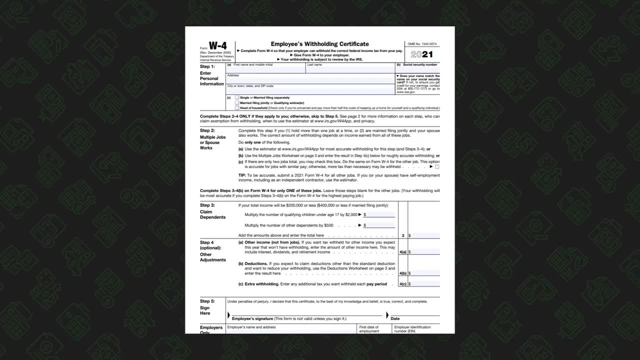 much taxes to withhold from the paycheck of the employee. It's required that all employees, whether full-time or part-time, complete a Form W-4.. Step number nine have the employee complete Form W-4.. Form W-4 is used, so you know how. 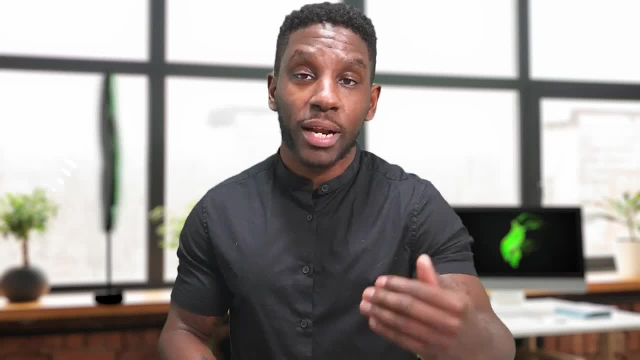 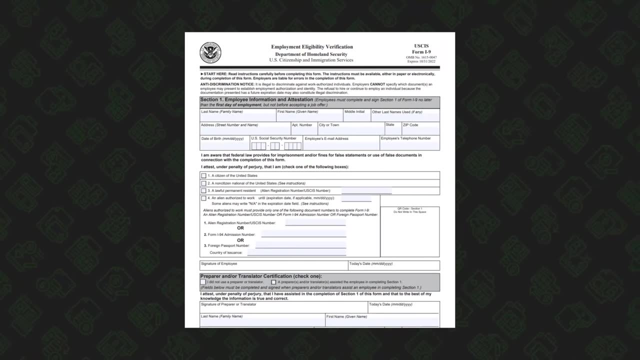 many taxes to withhold from the paycheck of the employee. It's required that all people complete this process on a regular basis. Also, mandatory personnel email it to the employee for this process. Step number nine: do not notebook all scams a rainy day and make any deposit on pensions bank notes. 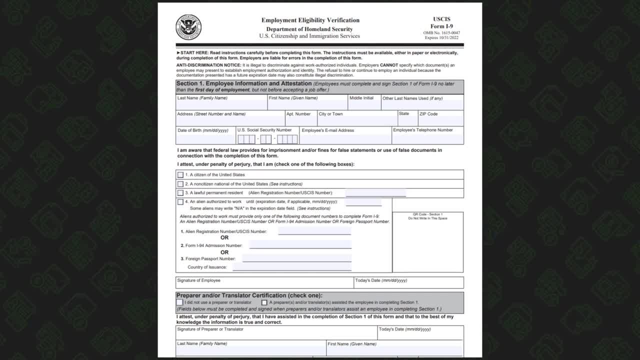 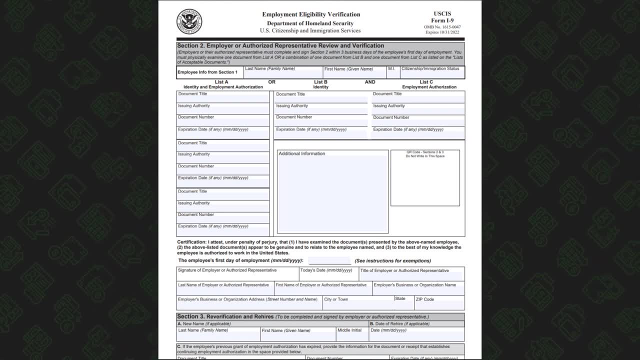 syndrome, shortcuts and bankGrand account. Each employee who has deployed questions to fill the form is required to fill the Form W-4.. Now a payroll service should include this step when onboarding a new employee. Step number 10, fill out Form I-9.. Form I-9 is used to verify the identity and employment authorization. 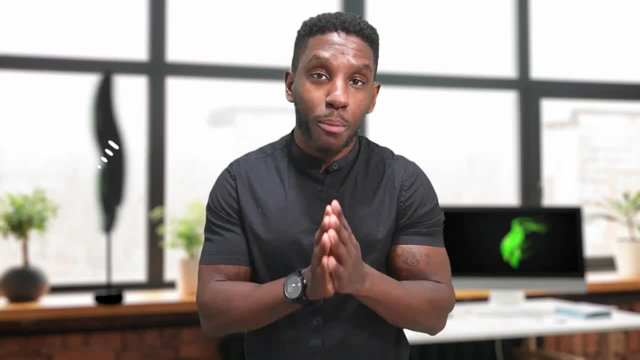 of employees that are hired in the United States. Each new employee must complete and sign the first section by the end of their first day. Employers must complete and sign the second section by each new employees' third day onboarding a new employee. Now, step number 11 is to remember important dates. Here are the: important IRS-related dates and tasks that I want you to remember. By January 31st you will need to send the IRS a W-2 form for each employee. By the end of February, you must send form W-2 to the Social Security Administration Within three days of hiring a new employee, complete form I-9 and. 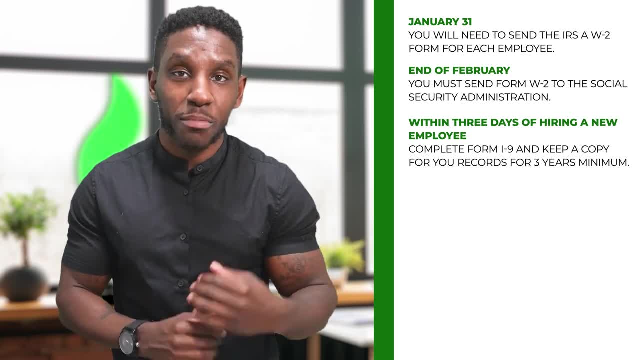 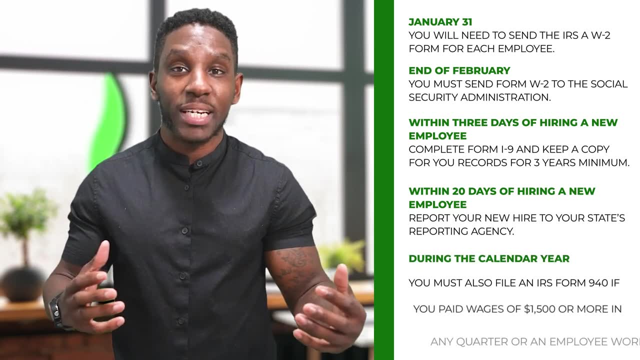 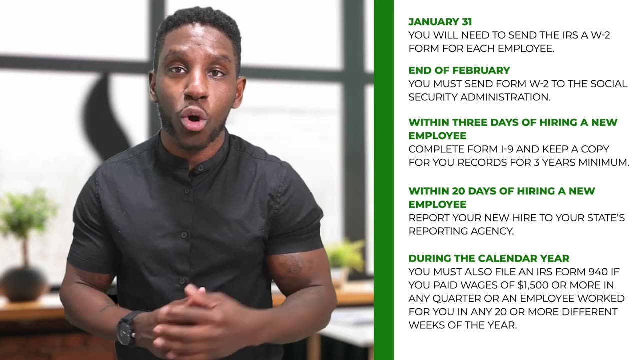 then keep a copy for your records for three years at a minimum. Within 20 days of hiring a new employee, report your new hire to the state's reporting agency, And sometime during the calendar year you must also file an IRS Form 940 if you paid wages of $1,500 or more in any quarter or 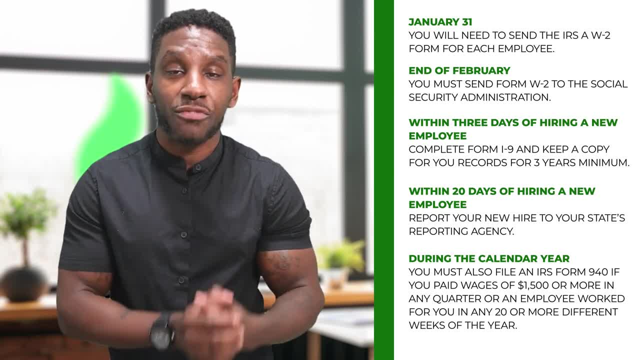 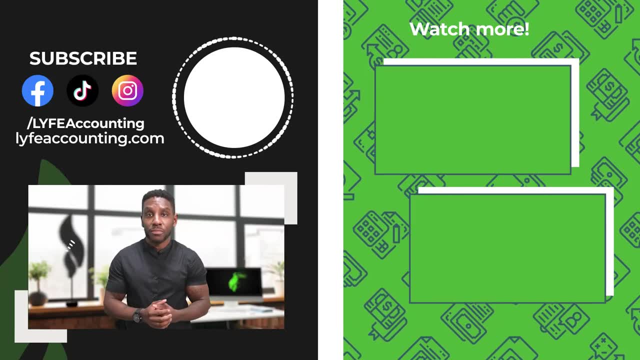 if an employee worked for you in any 20 or more different weeks of the year. I'm going to place a few videos on the screen I think you should watch. next, Be sure to check the out And if you found this video helpful, do me a favor. hit that like button for me. It helps. 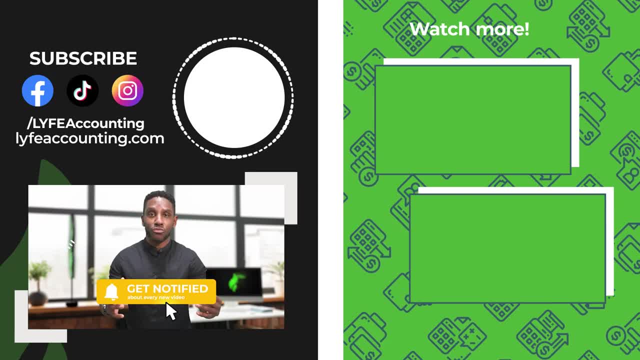 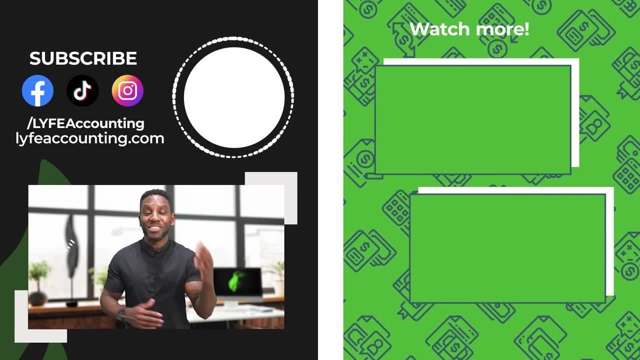 others to find this video on YouTube And subscribe to the channel for more financial information that helps you save on taxes and increase your wealth. I'm Karan from Life Accounting and I'll see you in the next video. 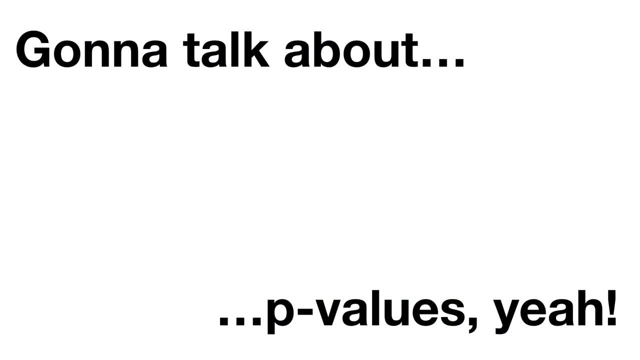 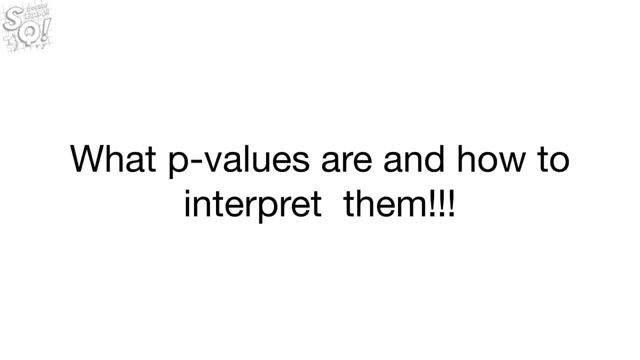 Gonna talk about p-values, yeah, StatQuest. Hello, I'm Josh Starmer and welcome to StatQuest. Today we're going to talk about what p-values are and how to interpret them. Imagine I have two drugs, drug A and drug B. 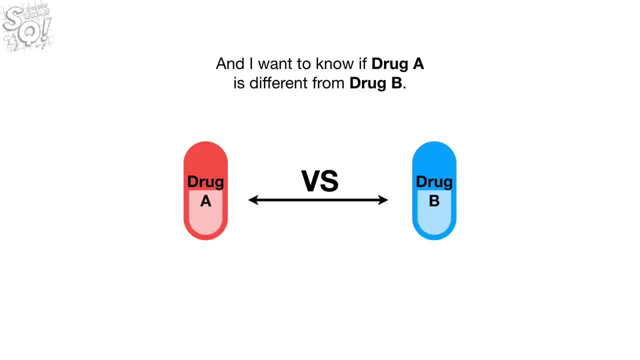 And I want to know if drug A is different from drug B. So I give one person drug A and I give one other person drug B. The one person using drug A is cured. Hooray. The one person using drug B is not cured. 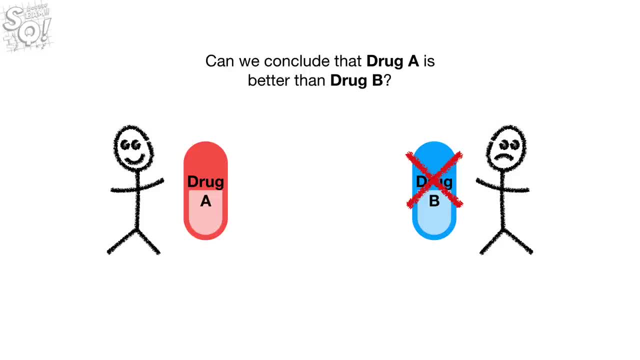 Bummer, Can we conclude that drug A is better than drug B? Nope, Drug B may have failed for a lot of people For a lot of different reasons. Maybe this guy is taking a medication that has a bad interaction with drug B.